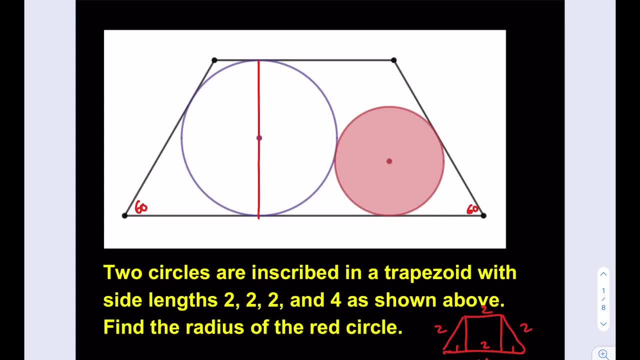 equal to the height of this triangle, right? If I go ahead and drop another perpendicular here I'm basically going to be getting. So we know that this is a 2 and this is 30 degrees, right, So we are actually faced with the shorter leg here. So, since this is, 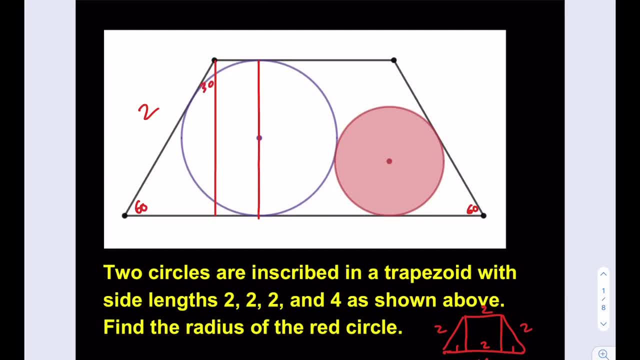 30 degrees. this should be 1,. right, This length should be 1.. Okay, awesome. Well, that means that the height is actually going to be twice the radius, right? So we can actually find the radius from here, because the height of this triangle is going to be twice the radius, right? 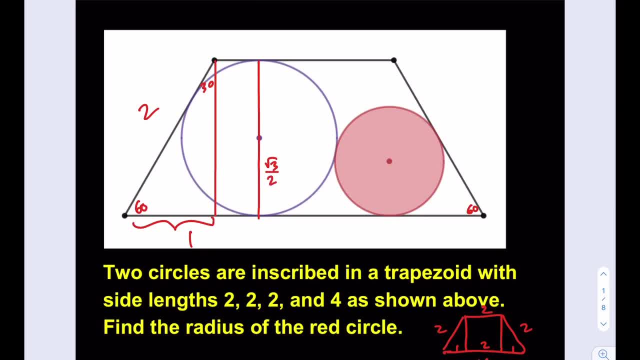 So this is going to be root 3 over 2, right. And this is going to be root 3 over 2, because the height needs to be root 3, correct, Awesome. What are we going to do from here? Well, we can just go ahead. 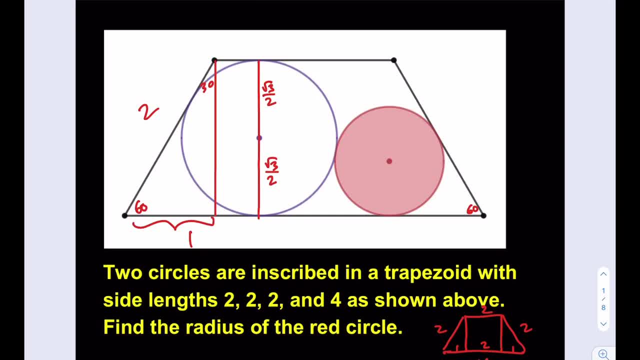 and proceed, but how do you find this length? That's another thing that we need to worry about, right? Well, here's what you can do. If you go ahead and make a connection here, like connect these two points okay, like this, you're going to notice that this is actually 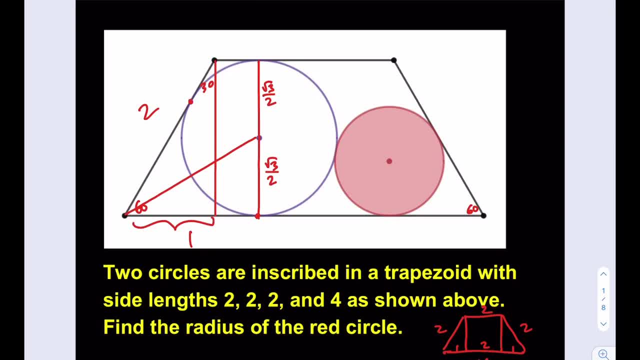 since this is perpendicular here, that's point of tangency. this is going to be 30 degrees and 30 degrees, So it's going to split up. Well, that means that if this is root 3 over 2, that's the. 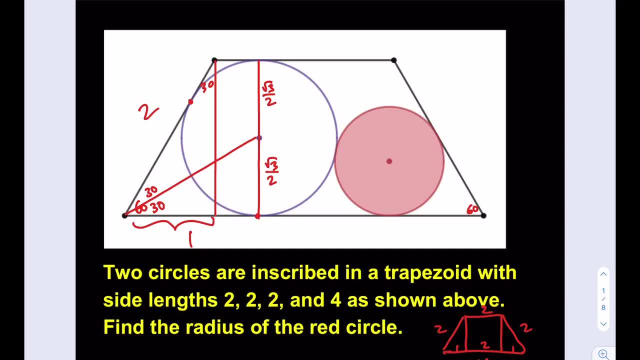 shorter leg right. Then the longer leg is going to be root 3 times that, which is 3 halves. So this length is going to be 1 half, basically right, Okay, awesome. So we know now that this length is 3 over 2.. Let's go ahead and make more connections here, For example: 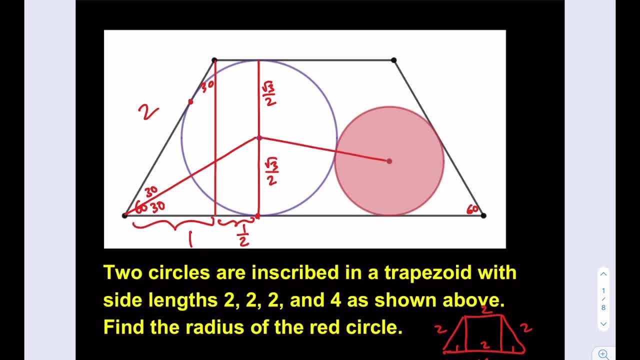 I can just go ahead and connect the centers here right And then drop another perpendicular- which will be helpful, right, And then also make this connection All right. so we also know that that's a 60 degree angle. so it's going to be split up into 30 and 30. 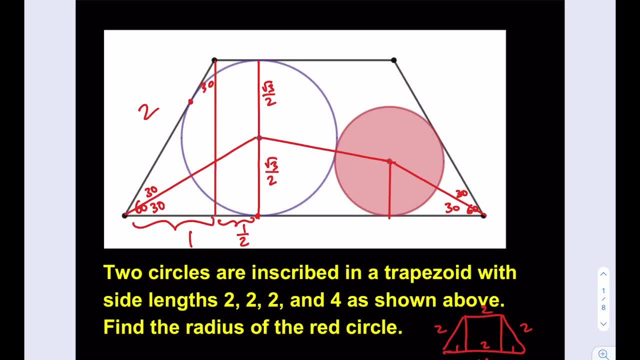 because we're getting two congruent triangles here at the point of tangencies. Okay, awesome. Now what do we know? We know that this length here, from this point to this point, is 3 halves. That's kind of cool, right. And we don't know the radius, So let's call this radius r And what we can do here. 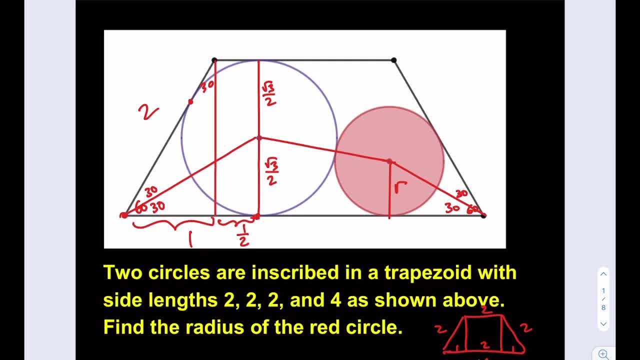 is. we can actually use the Pythagorean theorem. Let's go ahead and draw a horizontal segment here like this one, And then what we have here is. what we have here is: we know that this is going to be root 3 over 2 plus r. right, That's going to be the hypotenuse of this right triangle. okay, This right triangle here is going to have a hypotenuse of 3 over 2.. So we're going to have a hypotenuse of 3 over 2.. So we're going to have a hypotenuse of 3 over 2.. So we're going to have a. 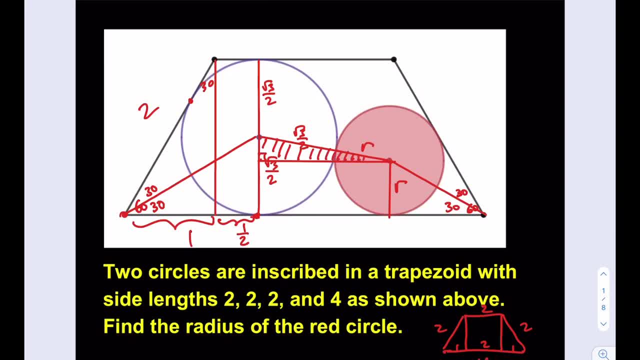 hypotenuse of root 3 over 2 plus r And the difference between these two lengths is going to be actually root 3 over 2 minus r. So this length is going to be root 3 over 2 minus r because we're subtracting them right. This is r, This is r. Okay, so we can actually find this. 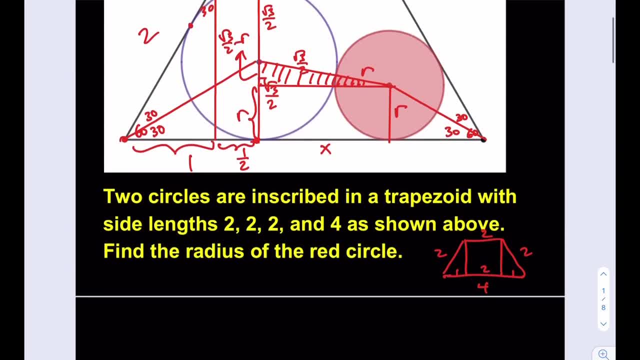 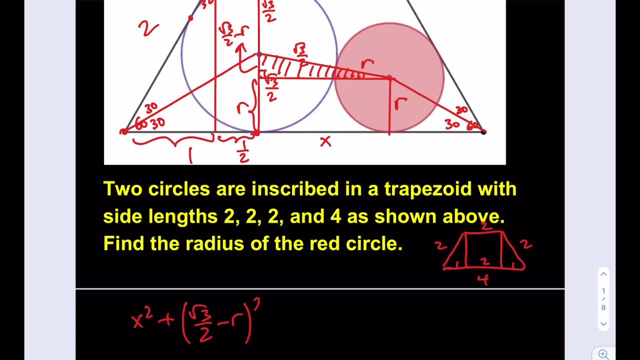 length. Let's go ahead and call that x. So what do we know? We know that from Pythagorean theorem. we know that x squared plus root 3 over 2 minus r squared is equal to root 3 over 2 plus r squared. But we just need another equation. obviously, right, Okay, but let's. 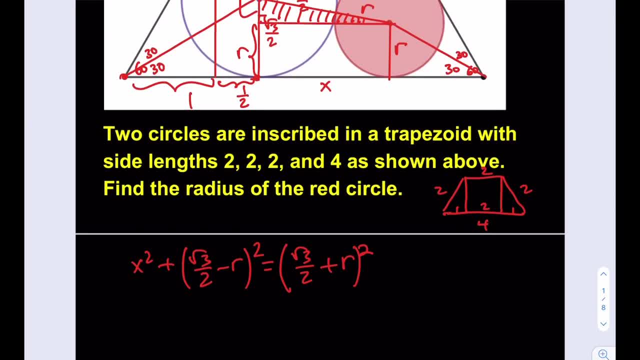 just go ahead and find x in terms of r here. So if I expand this- and you will hopefully remember the shortcut here- we said that if you subtract a plus b squared, minus a minus b squared, you get 4ab. So this is going to be 2 root 3r. So that's going to be the value of x squared. okay, And x. 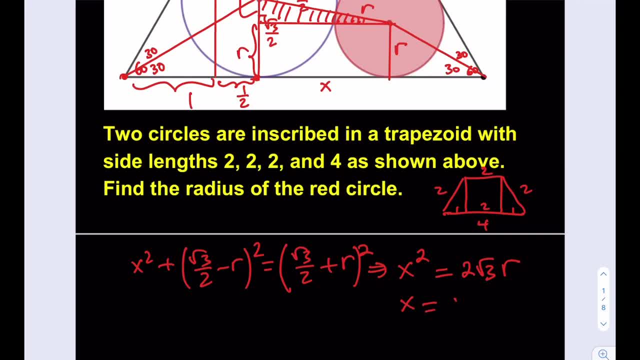 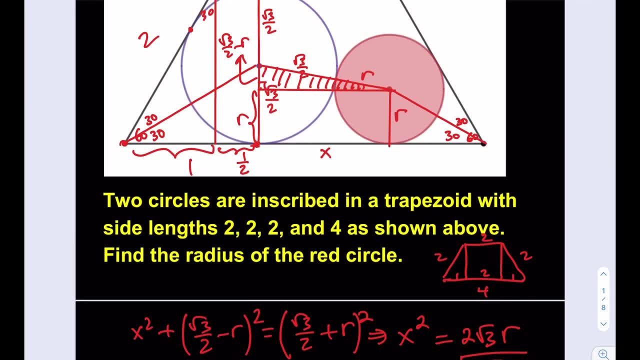 is obviously going to be the square root of that. So if you go ahead and do that, it's going to be the square root of 2 root 3r. So that's the value of x. here. We found that length, We know this length, So we got to find this length. Well, this is the longer. 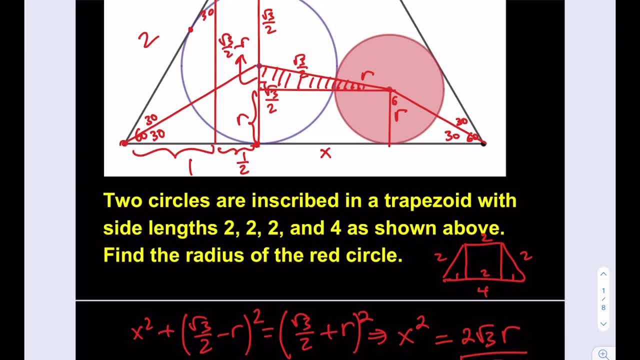 length in this 30-60-90 triangle, because this is 60 degrees. Therefore, this is going to be r root 3.. So, basically, I was able to get everything in terms of r: the base of the trapezoid, the lower. 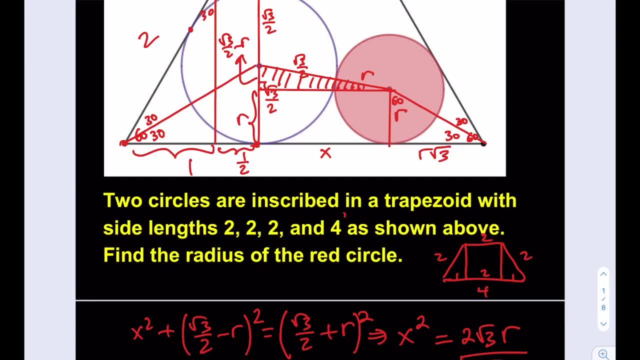 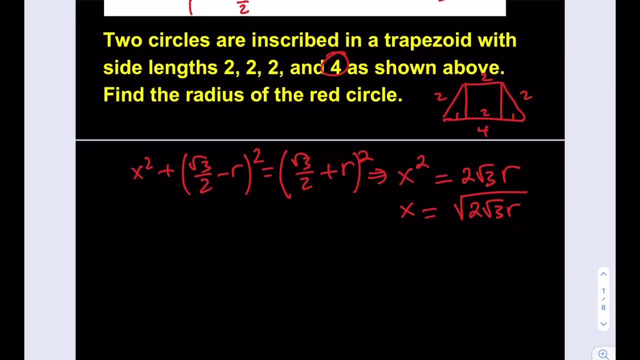 base, And we also know that it's equal to 4, because the lengths are given and all the other lengths are given to their congruence, So the lower base is going to be 4.. So now what we're going to do is: 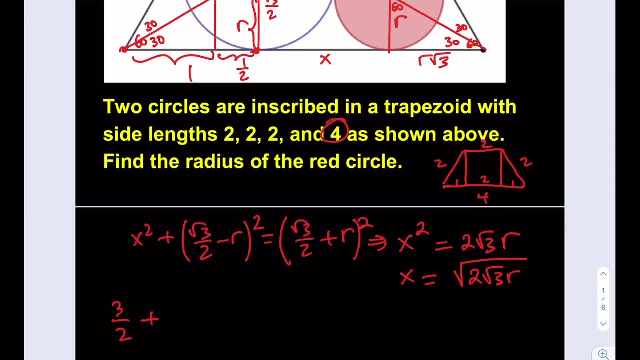 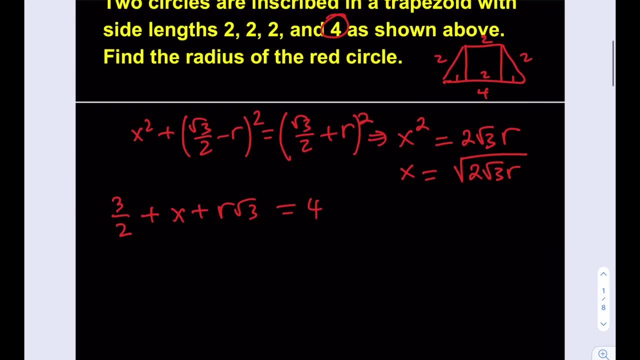 we're going to add those up: 3 halves plus x plus r root 3 is equal to 4.. Now I'm going to replace x with this value here, And I can actually go ahead and subtract some values. but it's okay, Let me go. 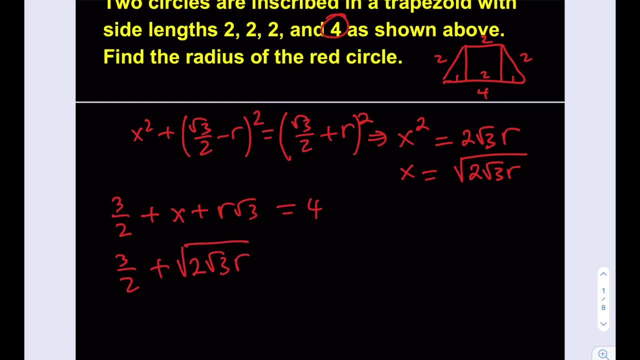 ahead and do this first, and then I'll show you what we're going to do. Okay, Plus r, root 3 is equal to 4.. Now what I'm going to do is because we have the square root of 3, we're going to do: 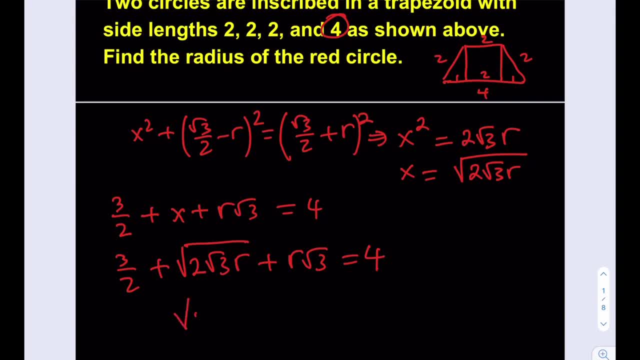 root of r. here I want to isolate that term. So let's go ahead and do that. I'm going to isolate it And everything else I'll subtract. So 4 minus 3 halves is going to be 5 halves, And then I'm. 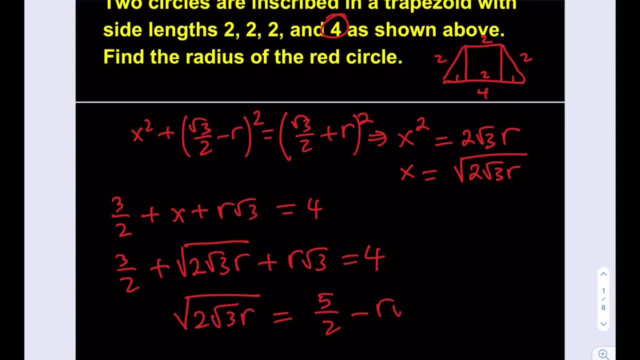 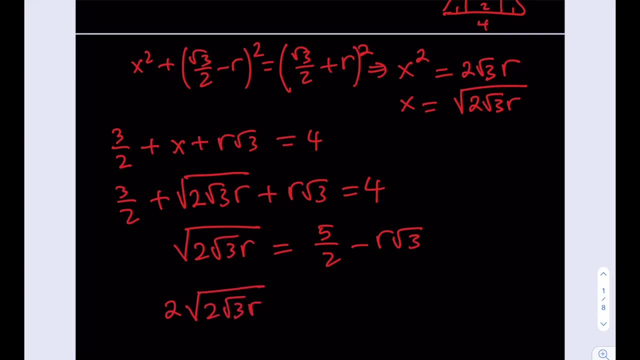 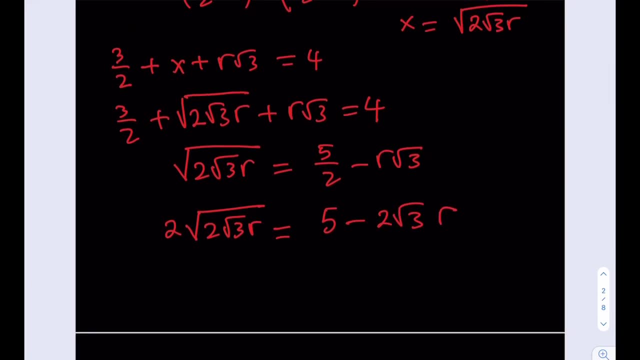 going to have minus r root 3.. And this is okay, because we're going to square both sides. So let's go ahead and multiply both sides by 2 first, before we actually square both sides. right, That's going to help And we're going to be getting this Now. let's go ahead, and let's go ahead and. 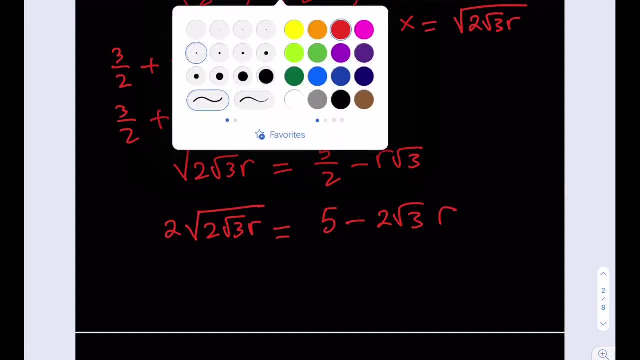 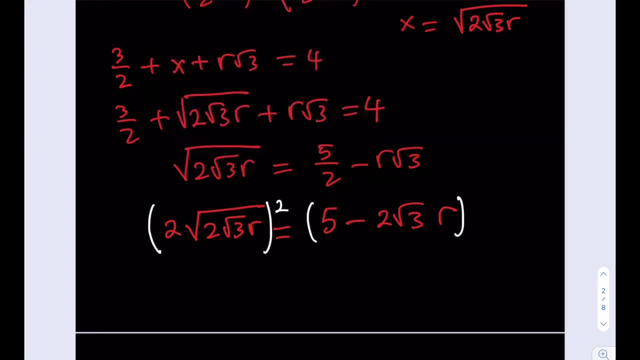 square both sides And once we square, we're going to be getting something nice, right? Okay, Let me go ahead and change it. Okay, So I'm going to go ahead and square both sides here And then let's see what happens. Okay, When you square this, you're going to get 4 times. 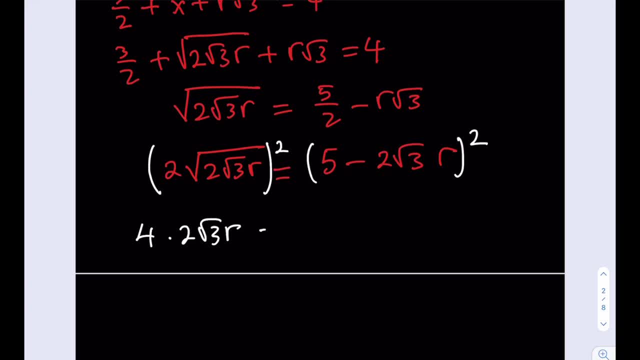 2 root 3r, The radical is going to disappear And the right-hand side- you're going to have 25 minus 20 root 3r plus 12r squared. Awesome. Now, if you go ahead and arrange these terms, 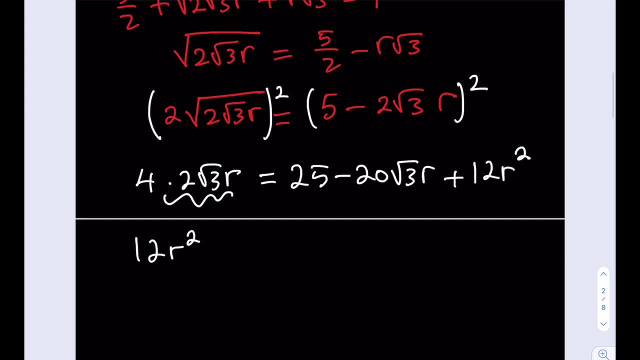 we will get 12.. r squared, This is going to be 8 root 3r. If I subtract it, I'm going to get minus 28 root 3r. plus 25 is equal to 0.. So what I need to do now is solve for r. Let's go ahead and do that. 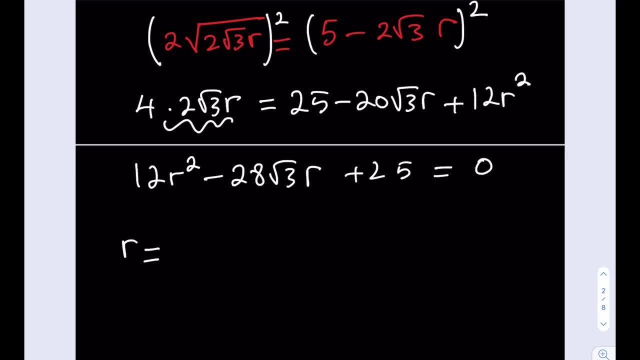 There is no common factor, so I can't really divide it. r is going to equal negative, b plus minus. We're going to decide which one is appropriate. The square root of b squared: Okay. This is kind of like a challenging one, So we kind of need to go ahead. 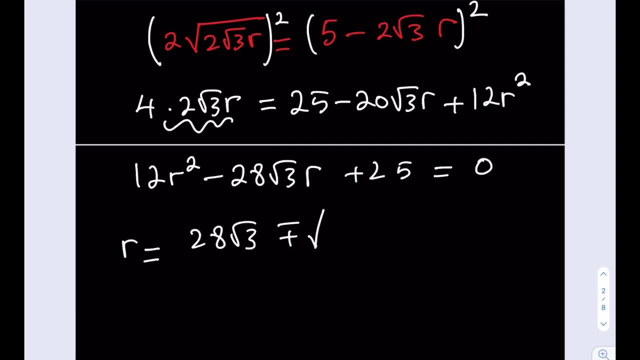 And square this. So it's going to be like 28 squared times 3.. And then b squared, That's b squared Minus 4 times a times c. So we're going to get something nice from here, because 4 times. 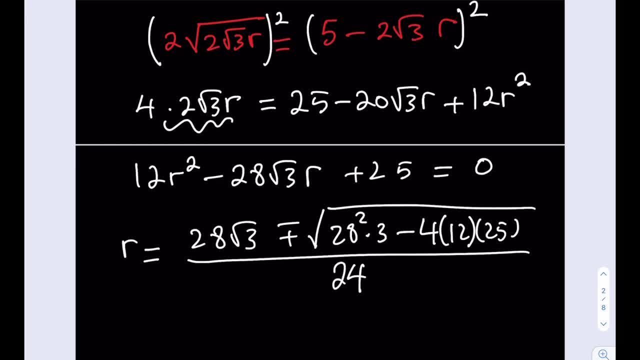 25 is equal to 100.. So that's going to be 1200.. Awesome, But we still need to calculate 28 squared. I'm going to tell you what it is in a little bit. Okay, 28 squared is going to be: 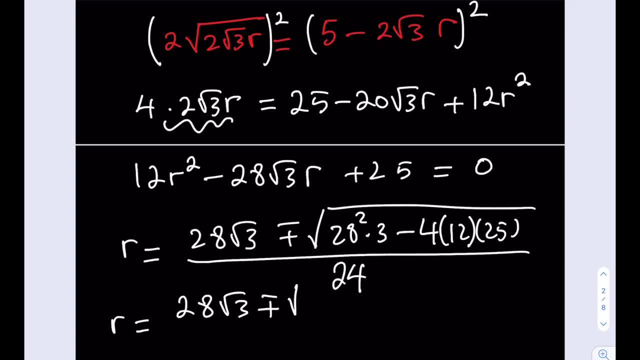 28 squared, So it's going to be 700.. Actually, let me go ahead and multiply that by 3.. So 8 squared multiplied by 3 is going to be hold on a second: 2352.. Okay, That's the value Minus 1200.. Okay, 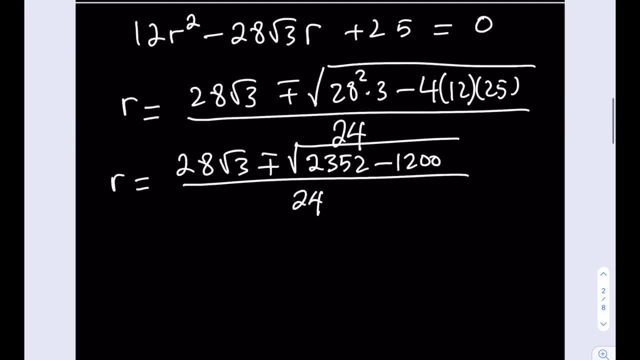 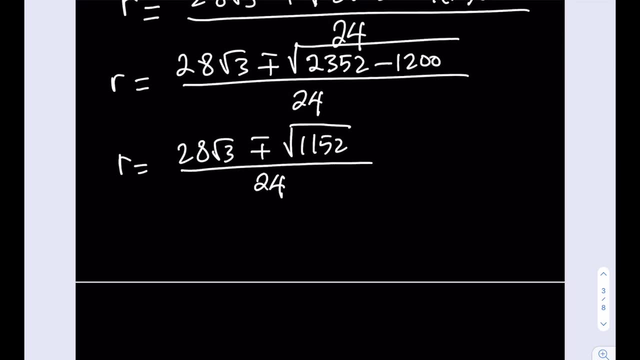 Let's see where this takes us. Very large numbers. So we get 28 root 3 plus minus. Okay, We're going to subtract and we're going to get 1152 from here. Let's go ahead and proceed. Now I got to simplify this number. How can I simplify it? Let's 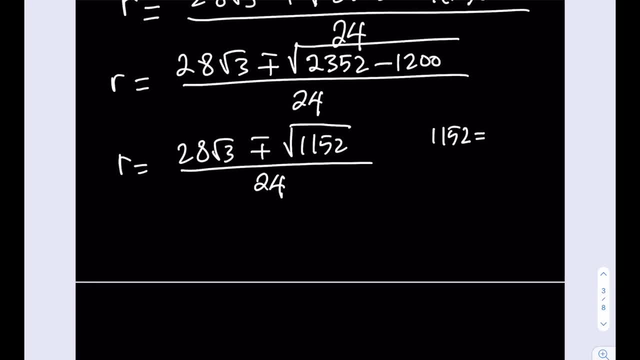 see if it contains any perfect squares. Okay, If I divide it by 2, that's actually going to give me 576.. Awesome, Isn't that? 24 squared, Beautiful. Okay, So that means the square root of 1152. 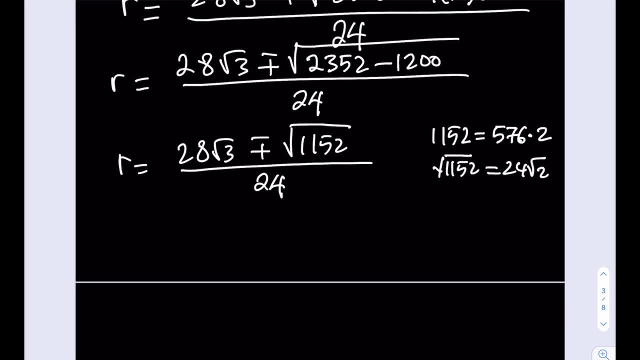 is actually going to be 24 root 2.. Awesome, So we can go ahead and write it as 28 root 3 plus minus 24.. Root 2 all over 24.. And obviously everything here can be divided by 4.. So so let's go ahead. 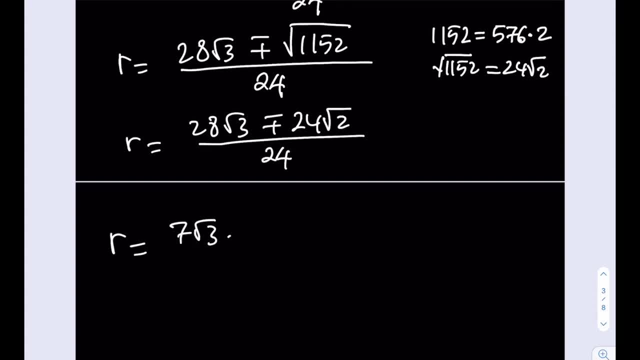 and do that. So that's going to give us 7 root 3 plus minus 6 root 2 divided by 6.. Now, at this point, you have to decide which one is appropriate. So let's go ahead and split them up, You might be. 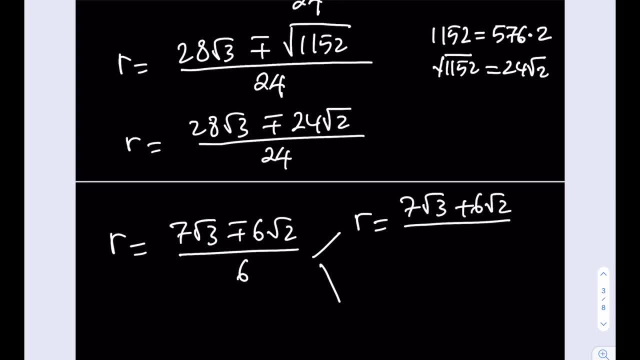 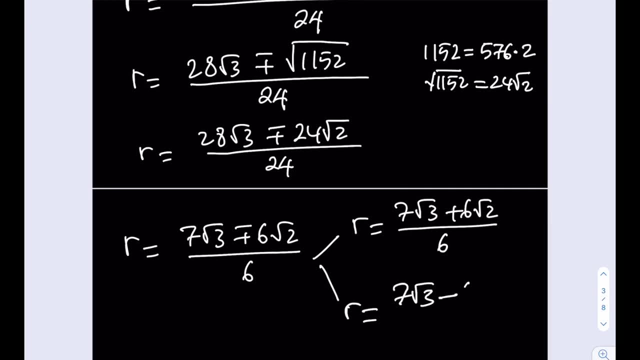 thinking like: oh, it should be positive, right, Because otherwise we may get a negative value. but obviously you're not going to get a negative value here because you're both positive And you knew that right When you got the equation from Vieta. Okay, Now 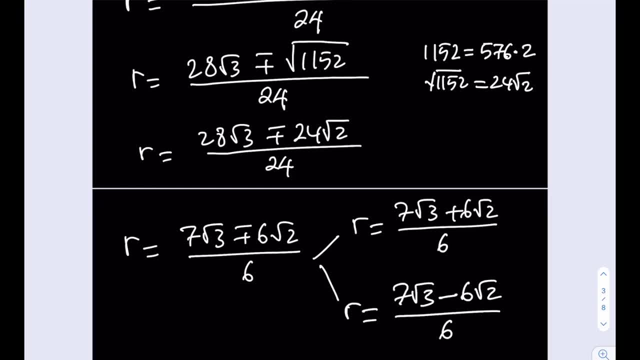 which one is appropriate. Now let's kind of try to estimate this. for, for example, the first one, right Root 3, is about 1.7.. If you multiply 1 point, let's say 1.6,, multiply by 7, you're going.